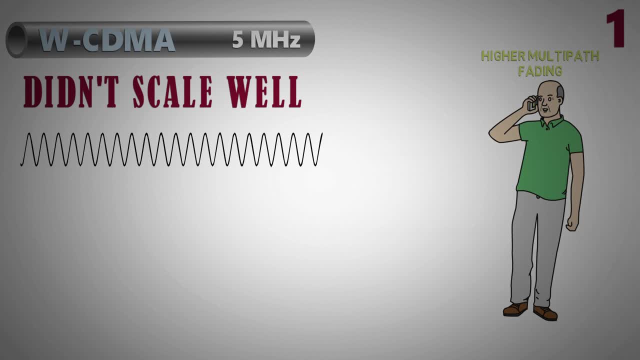 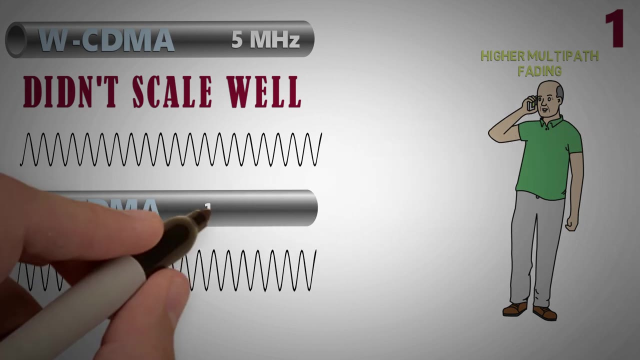 steps, which results in higher multipath fading. That's why Air Interface was redesigned and WCDMA was introduced, where, instead of spreading a signal over the entire band, the data is transmitted over many narrow bands of 180 kHz. As a result, the attainable data rate 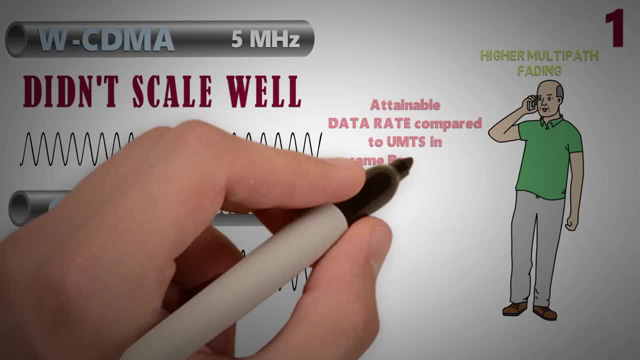 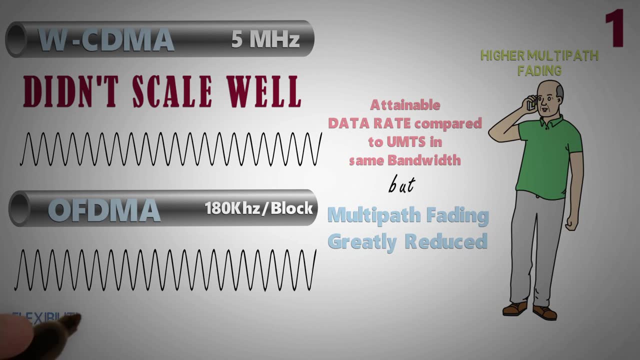 compared to UMTS is similar for same bandwidth, but multipath fading is greatly reduced. It also provides flexibility, as LTE can have bandwidth from 1.25 MHz to up to 20 MHz, and which can be further increased by carrier aggregation, thus providing more efficient. 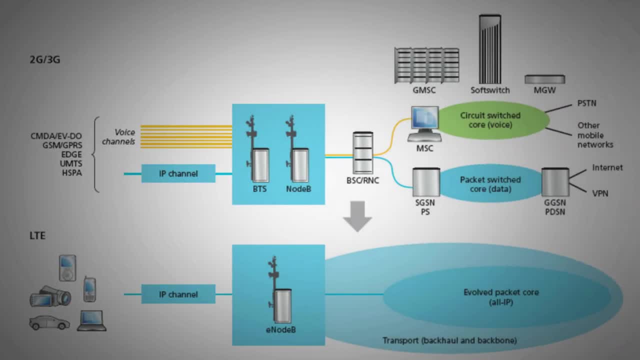 bandwidth utilization Now 2G or 3G uses traditional circuit-switched core for voice and SMS and package-switched core for data. That means operator has to maintain two core networks simultaneously. A major change in LTE was adoption of all IP-based core network, which means switching. 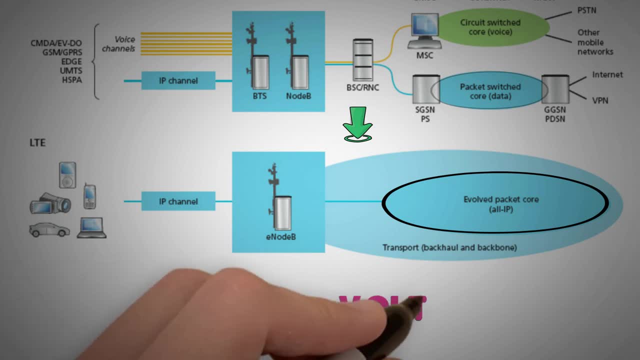 to VoIP or, in this case, IP-based network. It greatly simplifies the design and implementation of Air Interface radio network and core Quality of service mechanism on all interface ensures that bandwidth and other requirements of voice calls can be met even when the capacity limits are reached. 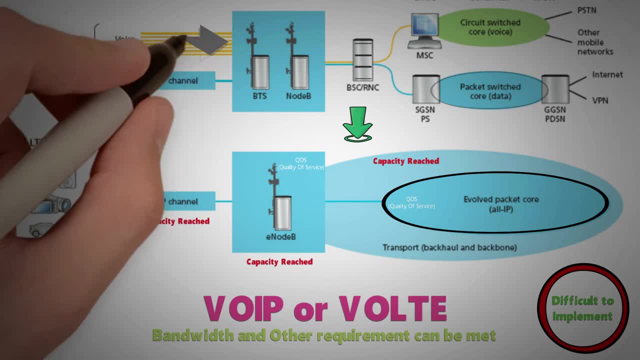 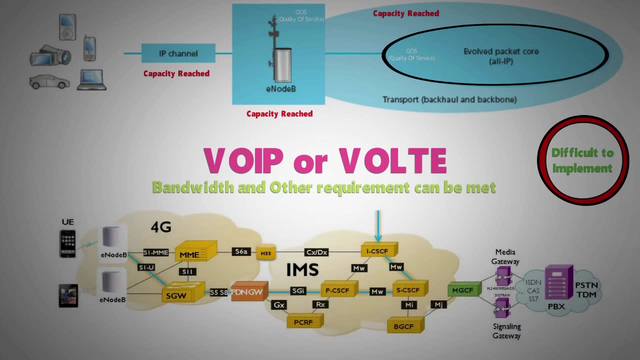 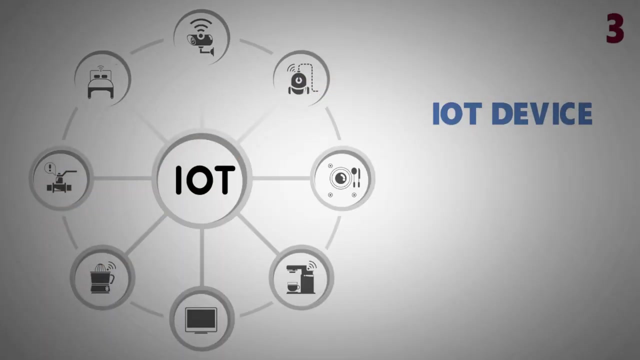 It is difficult to implement. that's why operators use circuit-switched fallback to 2G or 3G for voice calls. However, operators are migrating to voice-over LTE as it is cheaper and more versatile. With the advent of IoT devices, the total number of connected devices is expected to 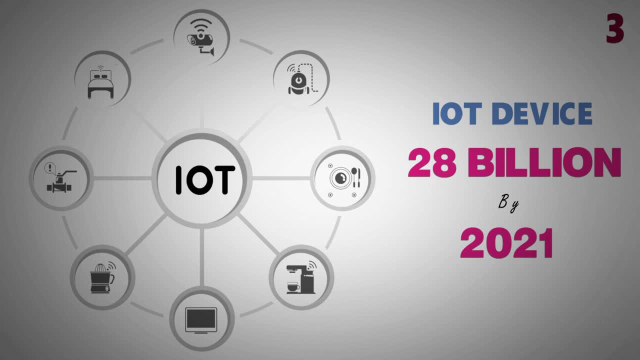 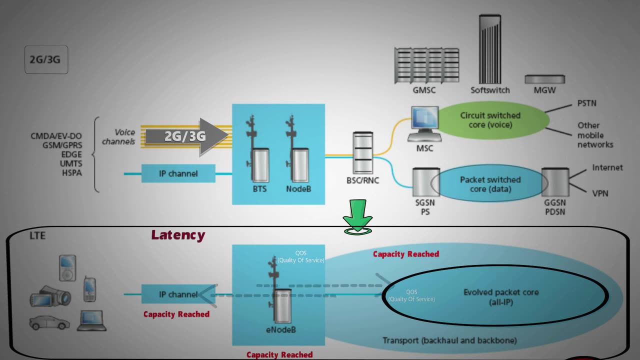 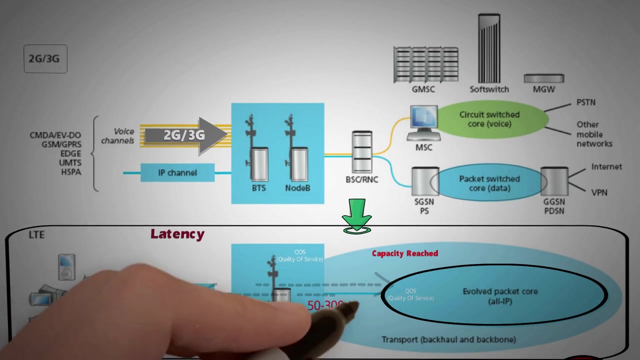 reach 28 billion by 2021.. Now, for these devices, latency is more important than bandwidth, so a faster backhaul was need of the hour. In LTE, the maximum allowed delay is of the range 50 milliseconds to 300 milliseconds. 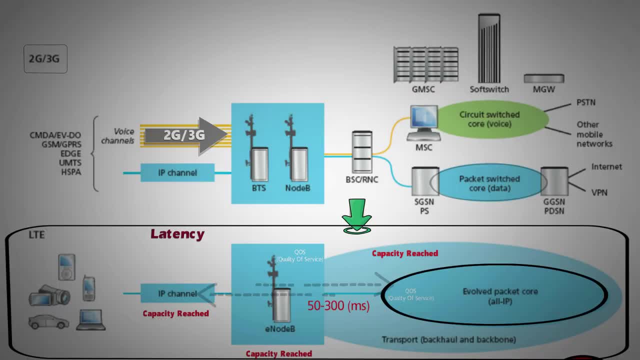 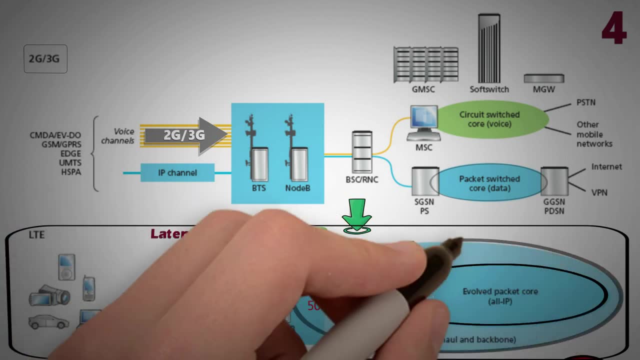 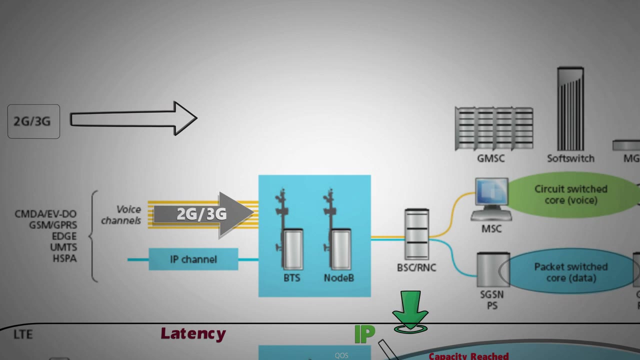 Also, all interfaces between network nodes in LTE are now based on IP, including the backhaul connection to the radio base stations. Again, this is a great simplification compared to earlier technologies that were initially based on E1, ATM and frame relay links, with most of them being narrowband and expensive.